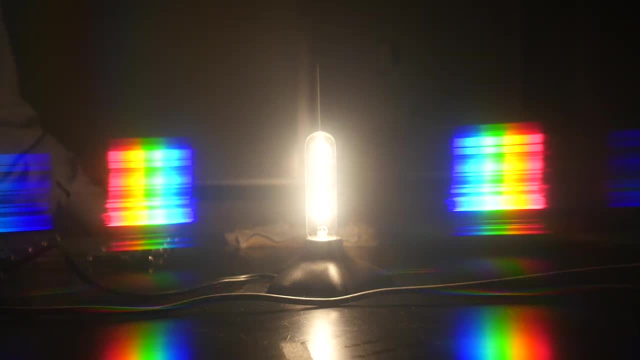 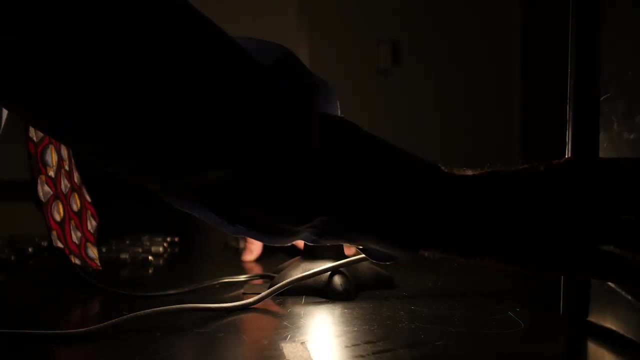 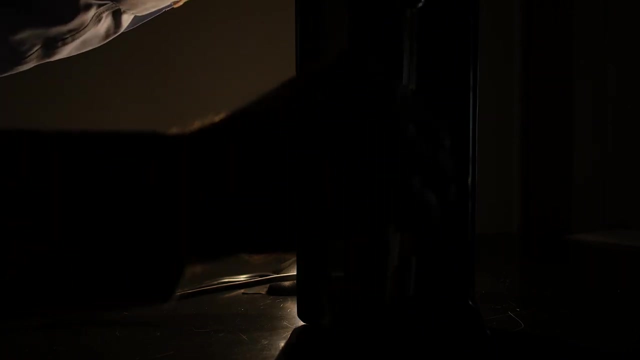 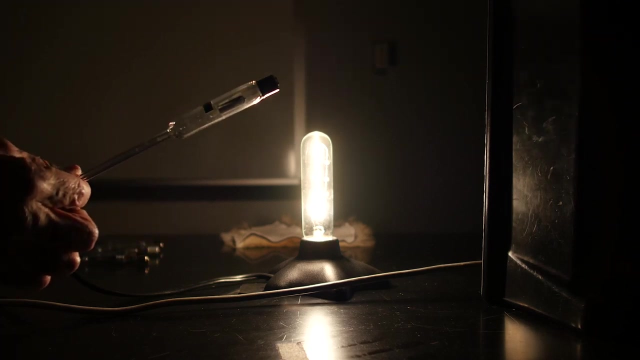 all the way through red. So that's a continuous spectrum. We'll try next to create. to look at a discrete spectrum of mercury. Now what this is? it's a discharge tube. It has mercury in it And what I'll do is energize this tube, apply a voltage to the tube. 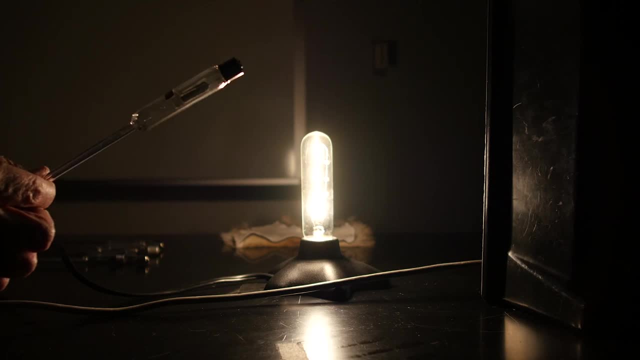 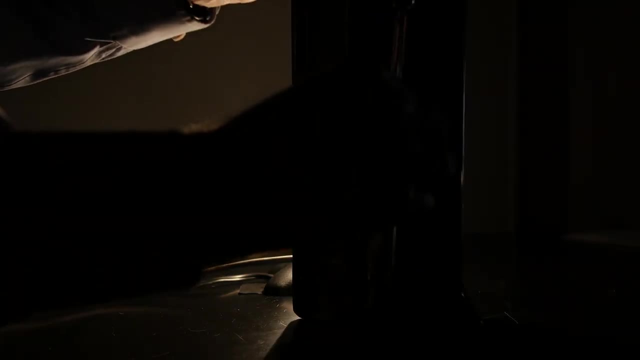 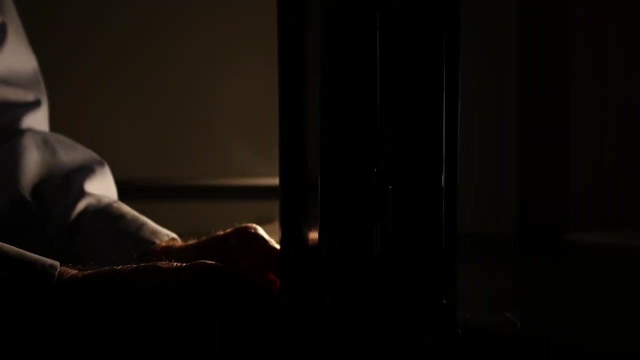 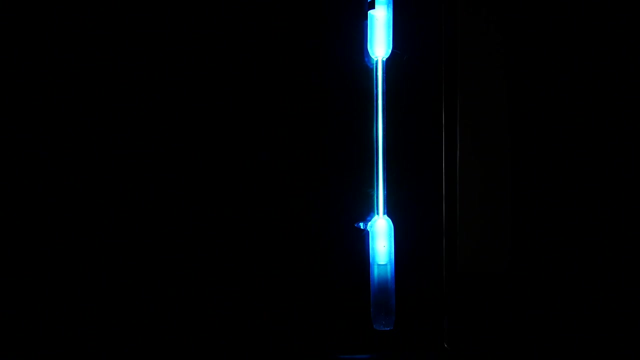 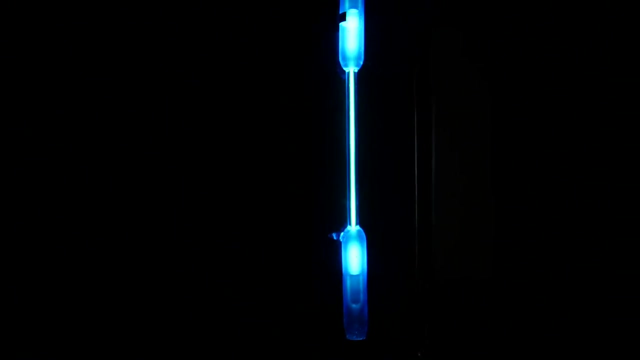 and that causes the gas in it to emit spectral lines according to the spectrum of the element that we're using, In this case mercury. So I'm going to locate this. It's a proper spot. Turn off the continuous spectrum. So this is a mercury spectrum without the diffraction grating. 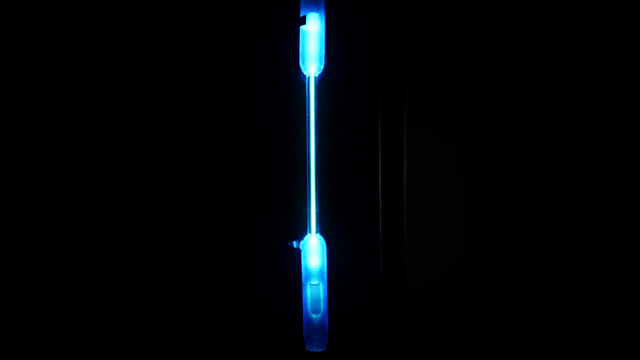 And let me get it in focus here. It's a bluish colored spectrum. There are mercury vapor lights that are used as street lights, So this may look similar to you, this bluish tint to the mercury vapor. Now let's try it with the diffraction grating in place. 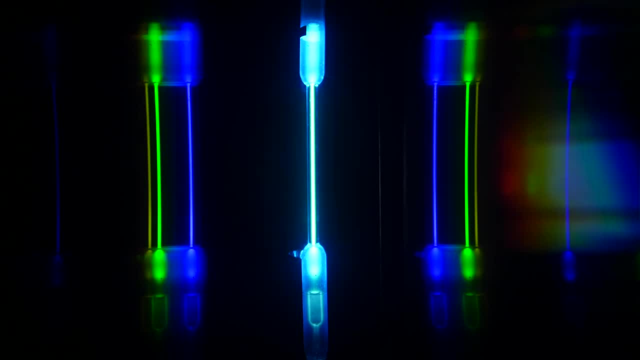 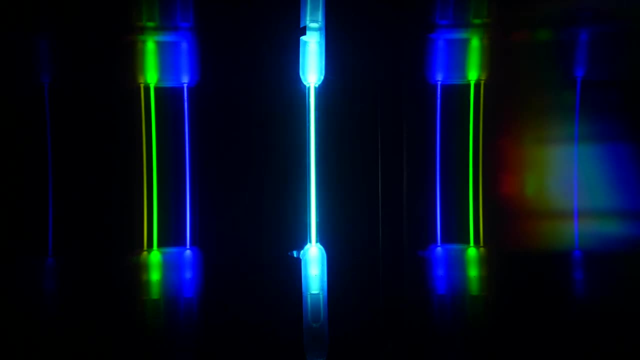 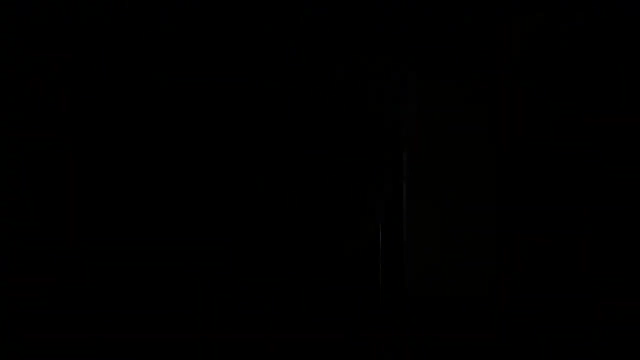 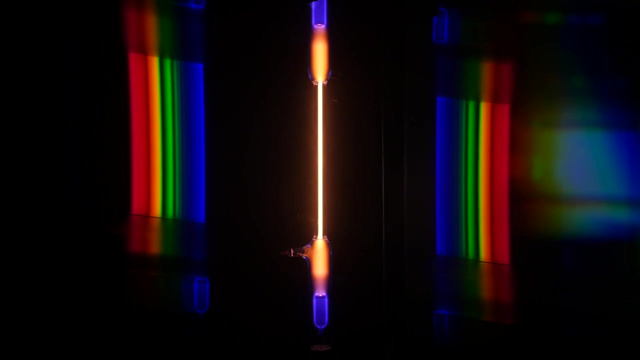 And what you see in this case are a green line and a blue line, predominantly in this mercury spectrum. Next, we will try a nitrogen spectrum. I'm using this fur to prevent burning flesh, So this is nitrogen spectrum And with the diffraction grating in place, we see a number of lines present. 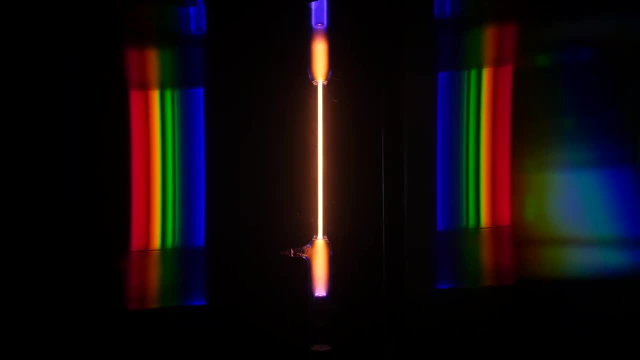 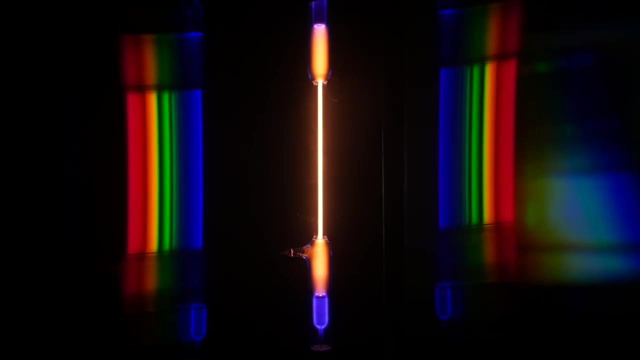 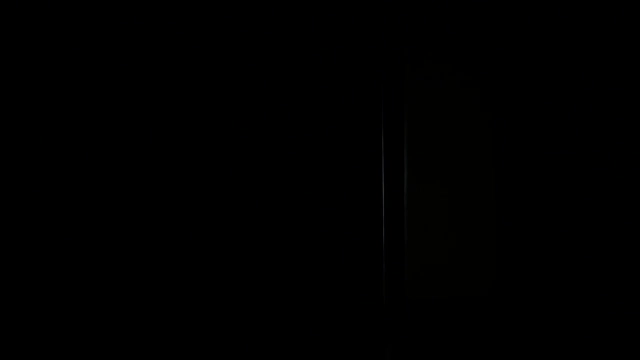 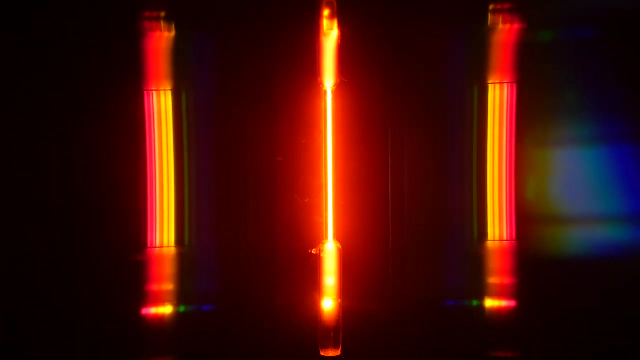 Some red, orange, yellow, green and a violet, turquoise-ish colored line. That's nitrogen. Two more: This is neon And there's a beautiful orange. look to it And when the diffraction grating is in place, you see a large number of red and orange lines.